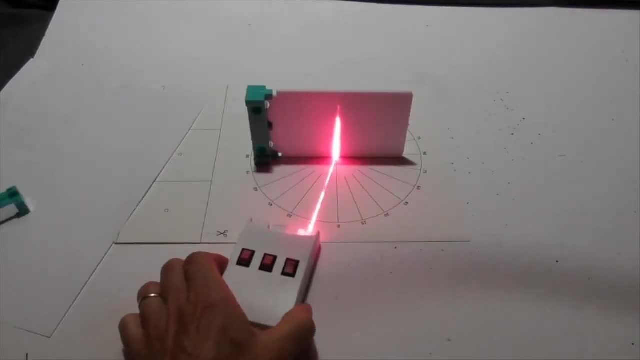 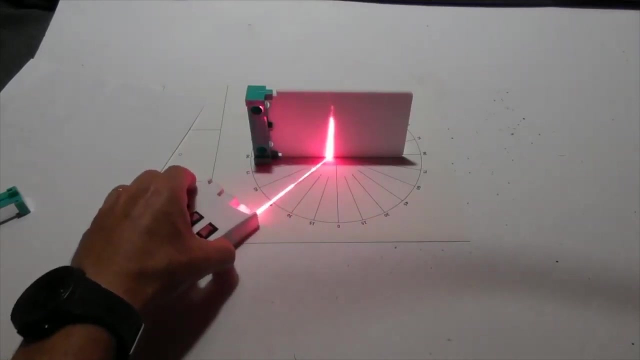 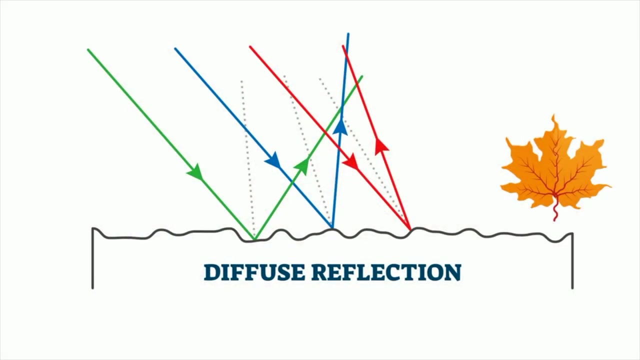 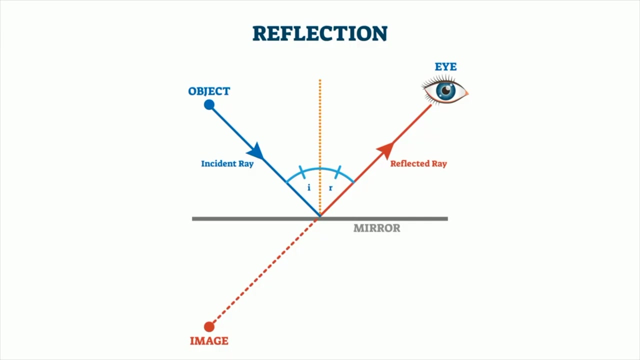 Next, I have a dull object: iosa 8920 ск. Reflection always looks the same, regardless of the angle. This is an example of diffuse reflection. During diffuse reflection, remember, the light is scattered in many different directions. With specular reflection, the law of reflection states that the angle of reflection of a ray 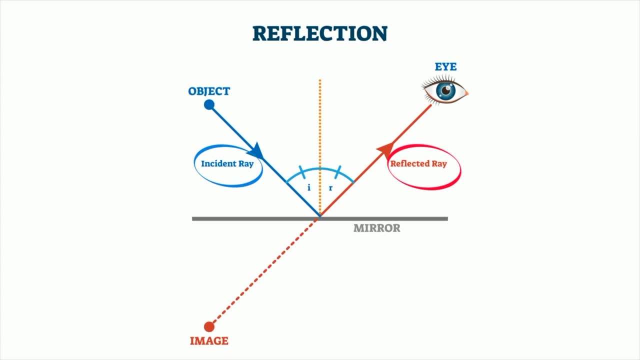 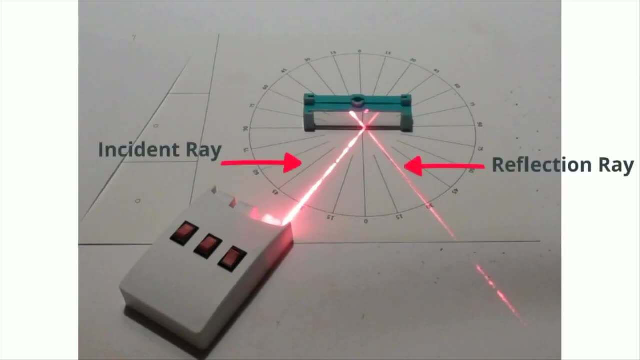 equals the angle of incidence. So lets identify a couple of items. Here's the ray of incidence, Here's the ray of reflection, And a line perpendicular to the surface is called the normal line, And again its perpendicular to the point where the light rays strike the surface. 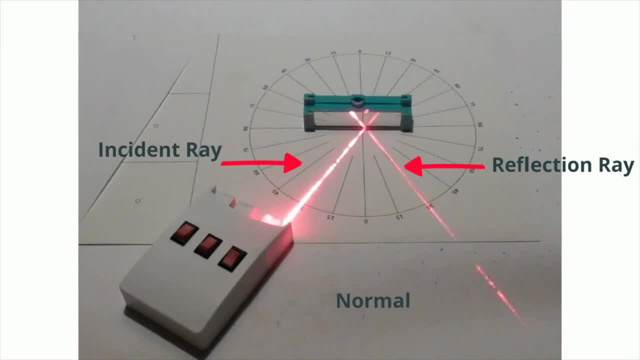 Also notice that at different angles you can see that the incidence and reflection are equal And you can measure these from the line of normal. Normal is at zero And the angle is at 30 degrees for both incidence and reflection. Here's another example. 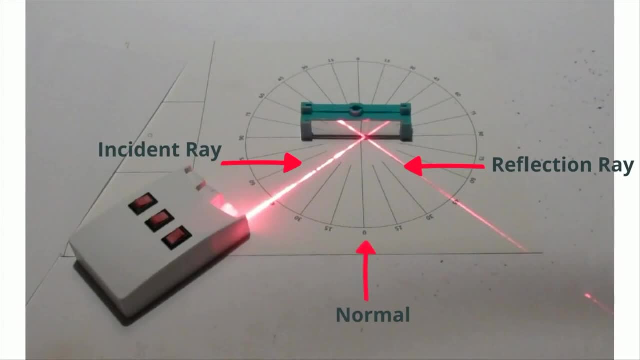 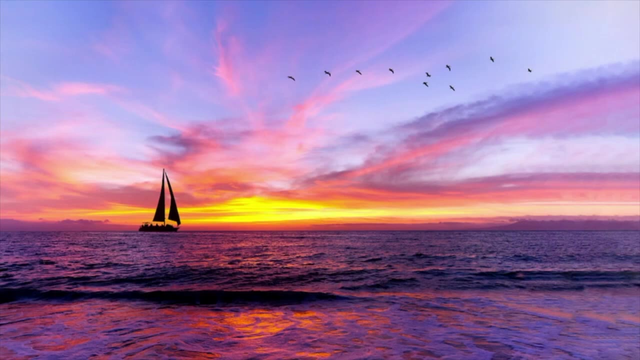 Normal is zero And incidence and reflection are at 45.. This rainbow and sunset are a result of refraction and diffraction. Welcome to MooMooMath and Science. Refraction is the bending of a wave when it enters a medium where its speed is equal to. 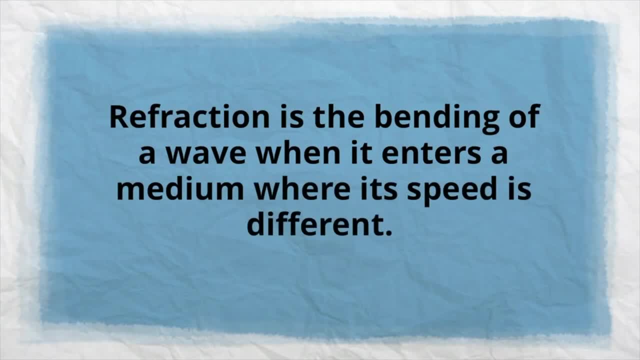 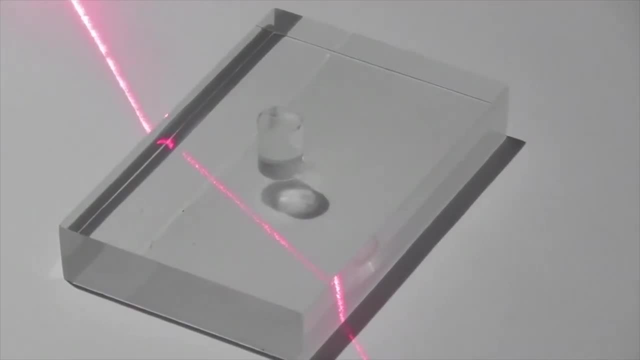 the speed of light Refraction is the bending of a wave. when it enters a medium where its speed is equal to the speed of light, The speed of light is different. For example, when this light enters this solid. you can see how it slows down and bends. 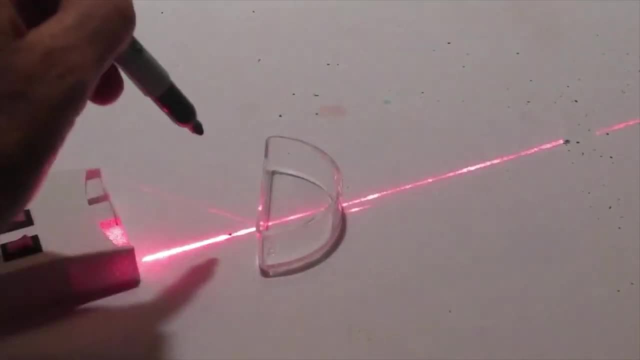 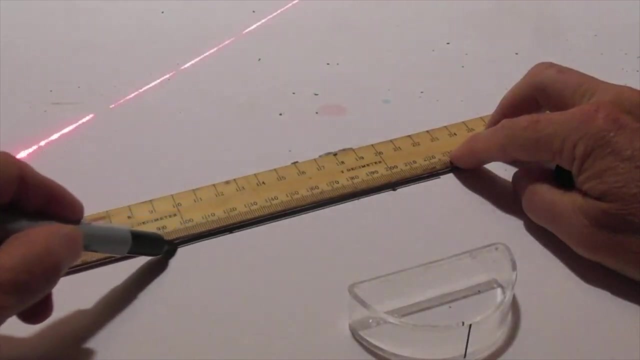 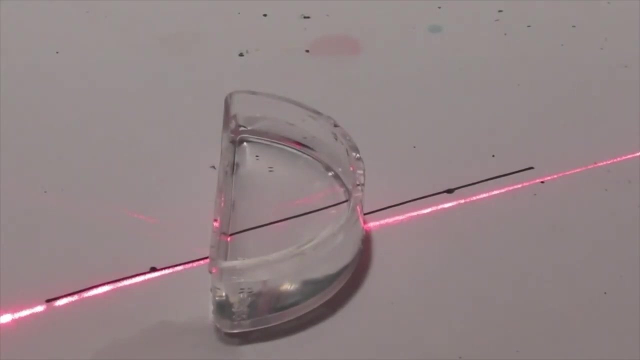 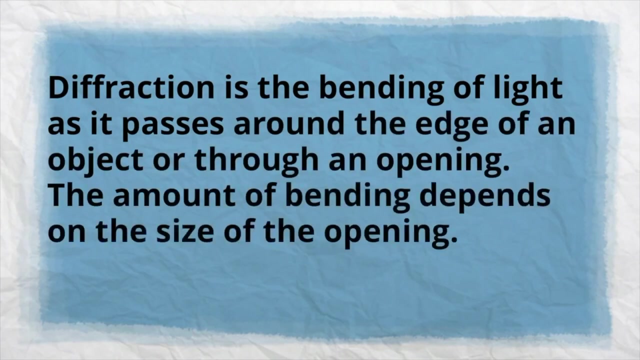 Next I have liquid. First I shine the light without the water inside. I mark it with my ruler and now, when I add water, notice how the light bends. It slows down and bends Defraction. It is the bending of light as it passes around the edge of an object or through an opening. 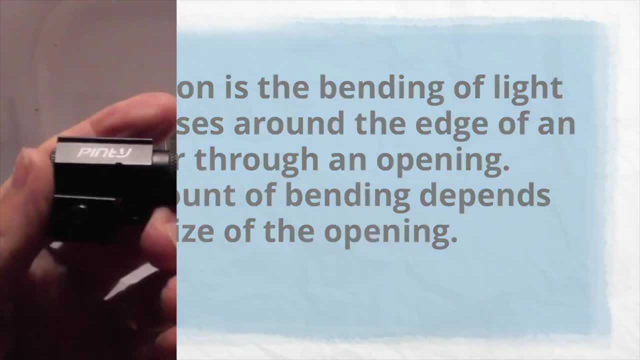 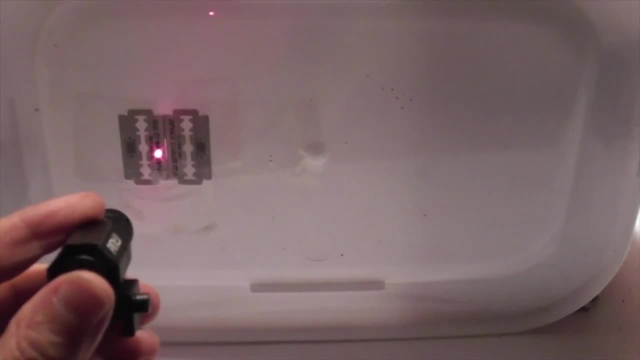 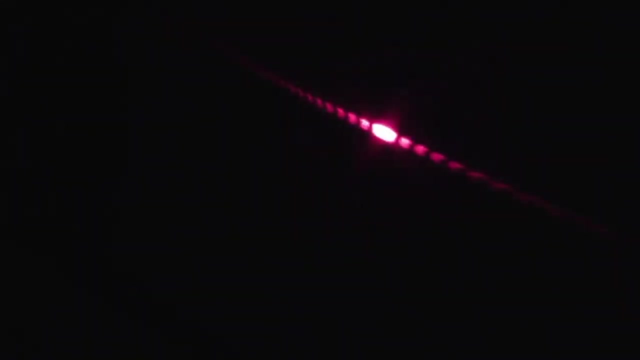 The amount of the bending depends on the size of the opening. What I did was I wanted to try to create a very small opening, so I got two razors and put them very close together and shone this laser through it. Now, here it is, with the lights on, and now you can see how dramatic it is when I turn.